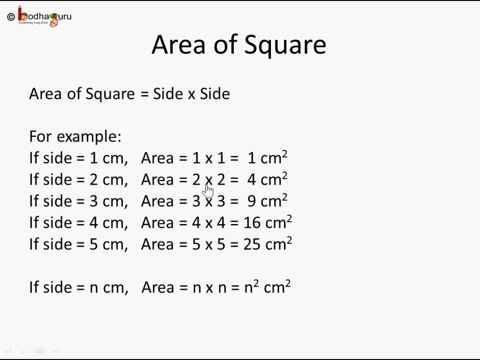 into one. that is one centimeter square. It's two centimeters. it's going to be two into two, that is four centimeter square. If the area of a square with side as five centimeter, the area would be five into five. that is, 25 centimeter square, or to put it generically: 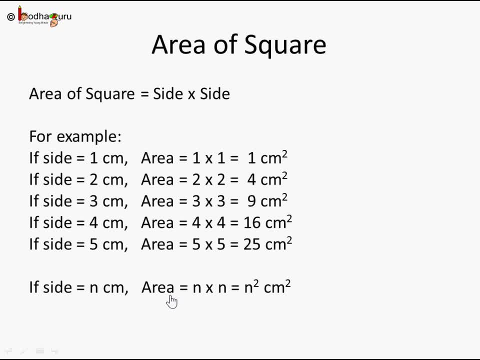 If there's a square with n centimeter as the sides, then its area would be n into n. let's call this n square centimeter square right, So 149.. What is this square? This square is 149.. Whatever we see here, 149, 1625, we can keep extending this. All these are known. 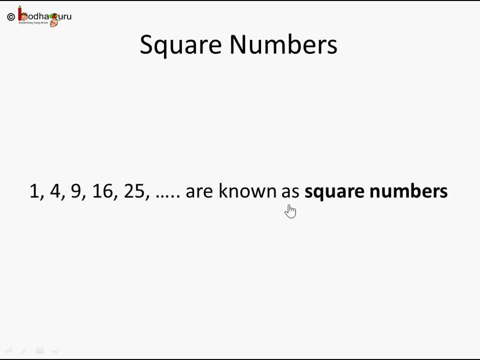 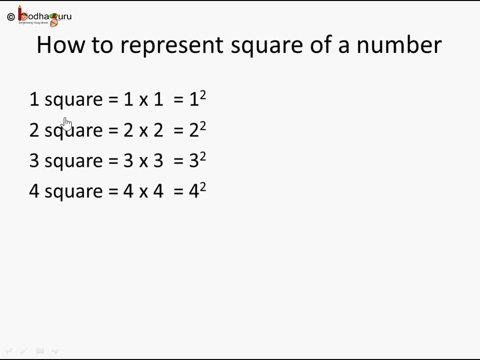 as square numbers, That is, it's a square of a number. So how do we represent a square of a number when we say one square, which really means one into one, that is a number by itself. one into one, it's represented one. 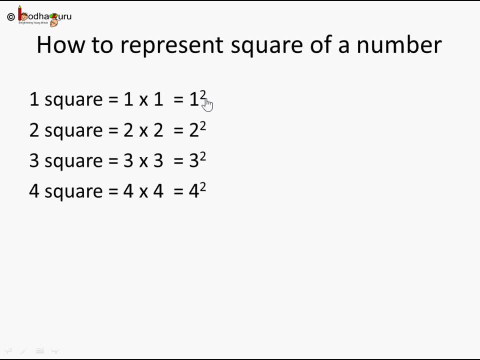 And we write two, A very small top left corner, in smaller size, two square. same way, two square means two as a number multiplied by itself. two into two, So it becomes two. then we write a small two, three square. three is the number multiplied by itself. three, small two at the top of it. 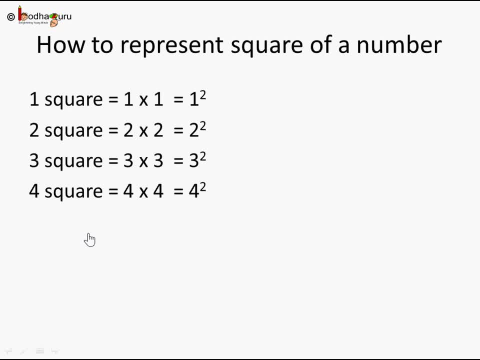 So to represent any number square, we just write that number like four and we write a two on top of it. That is That two, which is the, the, the power is saying four multiplied by four Makes sense. So we represent the square of a number by putting a small two on the top right. So now, 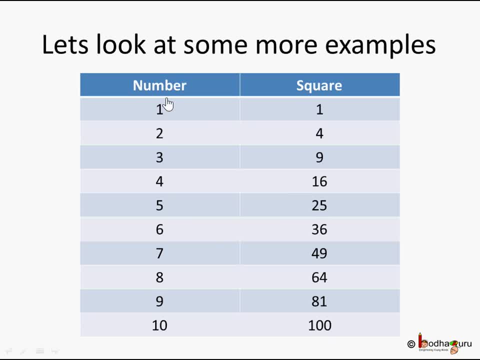 let's take some more example. On the left side I have certain numbers: One, two, three, four, five, six, seven, eight, nine, 10.. And right side, I have written it squares. Square means the same number multiplied by itself. 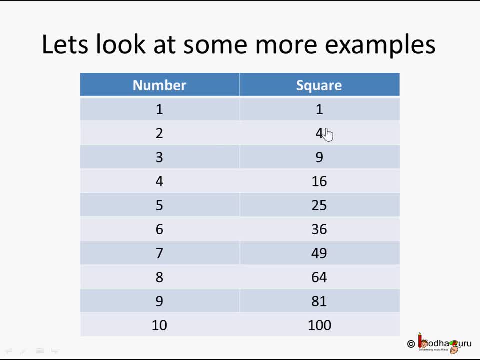 So one into one is one, two into two is four, three into three is nine, and so on. Eight into eight is 64,. nine into nine is 81, and 10 into 10 is a hundred, right? So let's look. 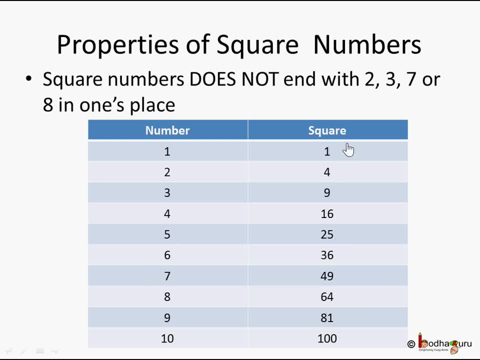 at certain properties of these square numbers. So here is a number and here are its squares. So if you observe all these squares, you will never find a square number. And, Okay, You will never find a square number ending with two or three or seven or eight in the 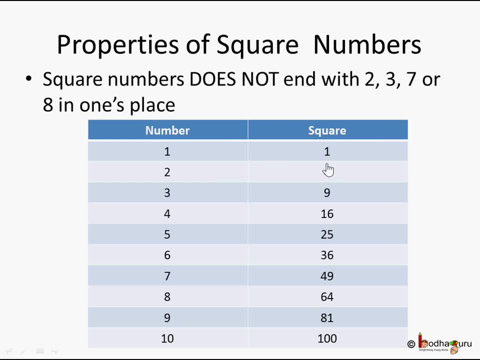 one's place. See, this is having one, This is having four, nine, six, five, again six, nine, four, one or zero. You will not find the squares ending with two or three or seven or eight. That is in one's place. You won't find this in the square numbers. You can keep. 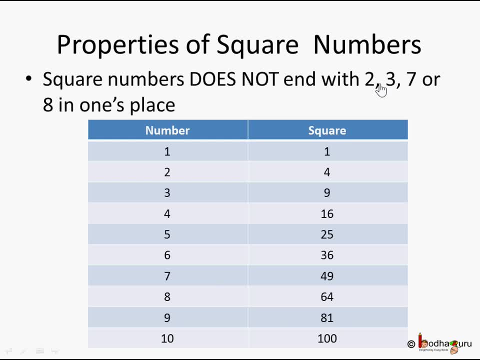 on doing for any number. You can take a big number Also. you will find other numbers, but not two, three, seven or one in the one's place. So this is one important property of a square number, If you are given. 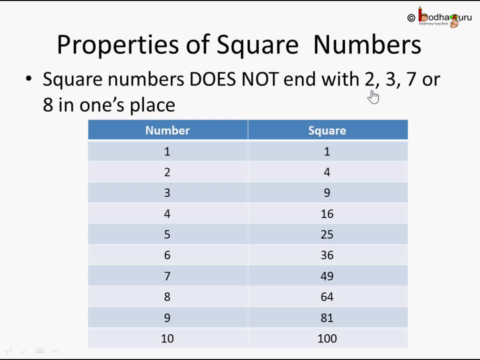 some sudden, suddenly a number one, 62,. you can say: is it a square number? That is, is it a square of some number? No, because it's ending with two. say I say three, 63, no, sending with three. So it cannot be a square number. 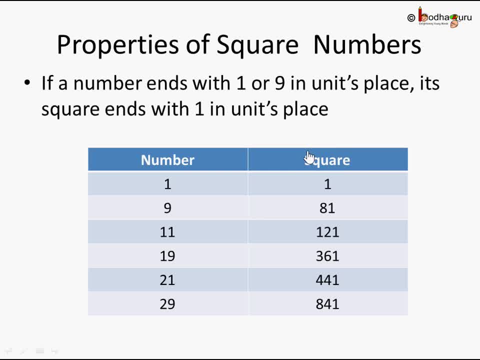 Let's look at another property. Okay, If a number ends with one or nine in units, place like here are: I've taken certain example number like one: nine, 11,, 19,, 21,, 29.. I can go 31,, 39,, four, 41, four, 49.. If a number 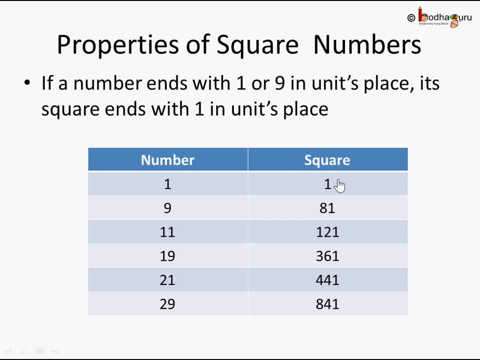 ends with one or nine in units place, then it's square always ends with one. Here you can see: 11 into 11 is 129.. Okay, 21,. 19 into 19 is 361.. So the squares are all ending with one. So if the number ends, 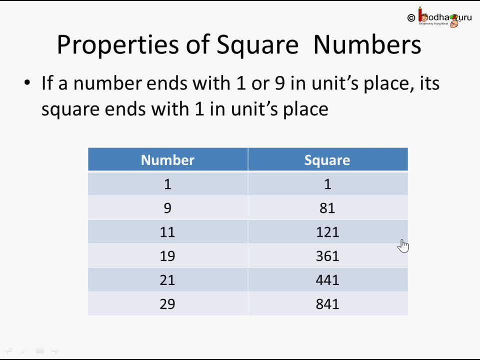 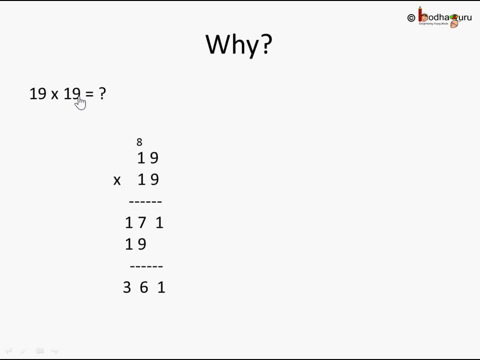 with one or nine square ends with one. why is it So? we know, just purely by the rules of multiplication. say, I take an example, 19 into 19.. So I write: how do we do two digit multiplication? We write 19 into 19, and then we do single digit at a time, right? So we 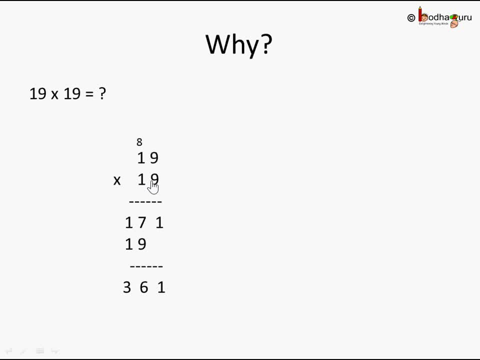 do nine into nine, 81,. then nine into one is nine plus eight is 17.. The next we leave it blank, or we can put X there or zero. Then we do one into nine, nine, one into one, one. then we sum it up. 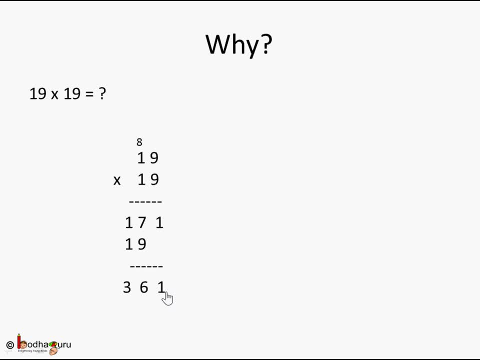 So when we do the sum, you see one plus zero is one and rest. you keep on doing. So if any number is ending with nines, then nine into nine is always 81. It can be a very big number, Okay. Also: two, three, five, nine into two, three, five, nine: always nine into nine will be. 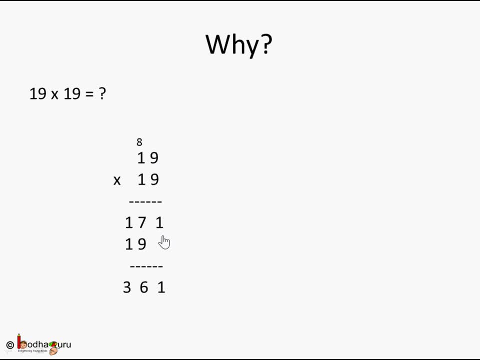 81. And in the next step there will be zeros here. So when you add them it will always be one. Exactly the same thing holds true for ones. So suppose the number was 21 into 21,. one into one will be one, And that is the reason. any number which is ending with 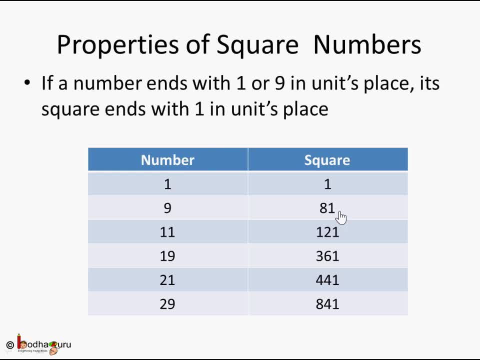 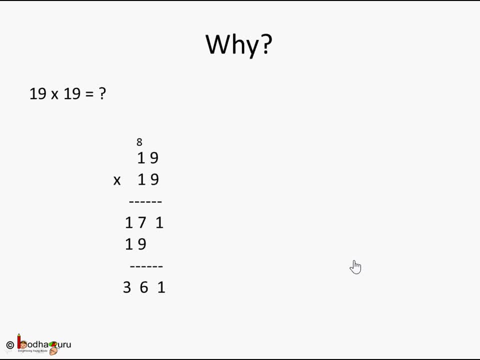 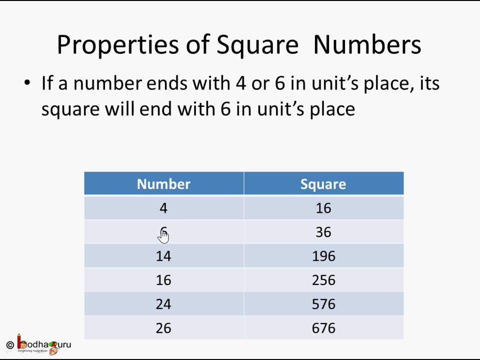 one or nine in their ones place, We'll always be having one in their squares place. Make sense. Let's take another property on similar lines. If a number ends with four or six, then it's squares always ends with six. As you can see here, 26 into 26 is 676.. 24 into 24 is 576.. And why is that? Because 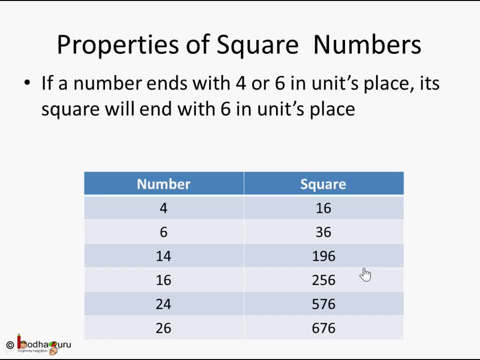 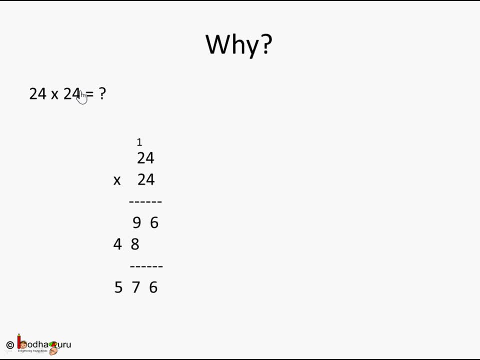 Again, do a simple multiplication and you'll know why it's that case. Let's take 24 into 24.. Just do a normal two digit multiplication. How do you do? Just do the first step. Four into four is going to be 16.. So six will come here and one will go and carry over And in. 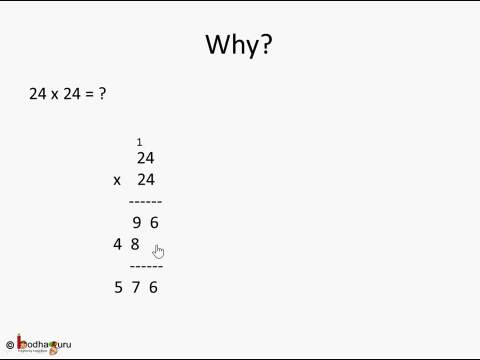 the second step. there won't be any number here. it will be blank or zero here. So six plus zero will be six. So the ones place in this square number, that is 24 into 24 product, will always be six, 6. if I take a big number, 3, 2, 5, 7, 4 into 3, 2, 5, 7, 4 in the ones place in the 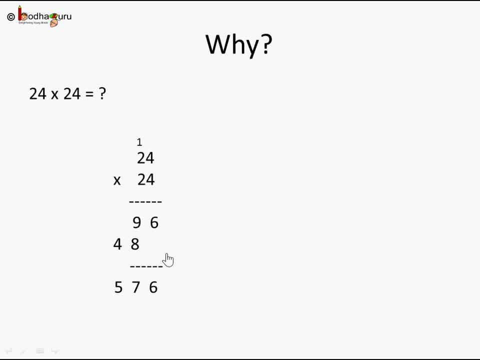 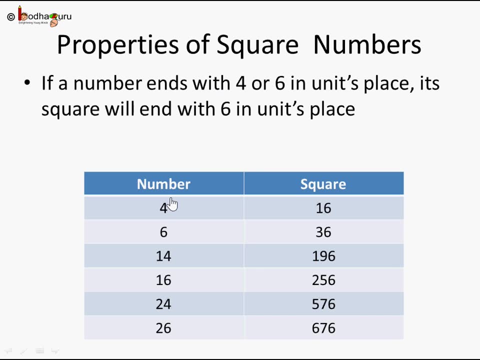 product will be a 6, because 4 into 4 is a 16 and 6 you write here and 1 goes somewhere in the top. rest of the numbers can be in anything. but the property is saying: if the number ends with 4 or 6 in the units place, then its square will end. 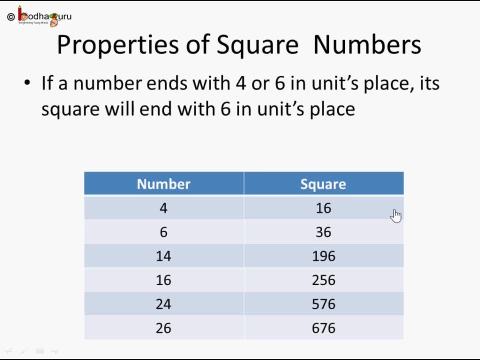 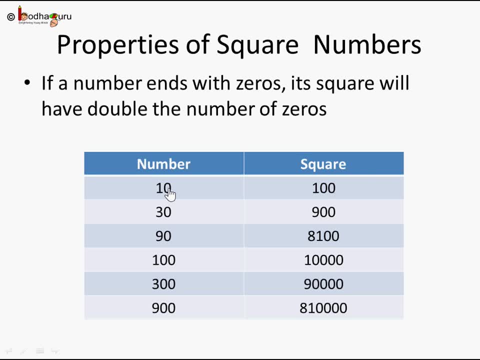 with 6 in the units place make sense. one more property: the number ends with 0, then a square will have the double number of zeros. what does it mean? let's take an example: 10 into 10 is 100, so it ends with 1, 0 and in the square you see. 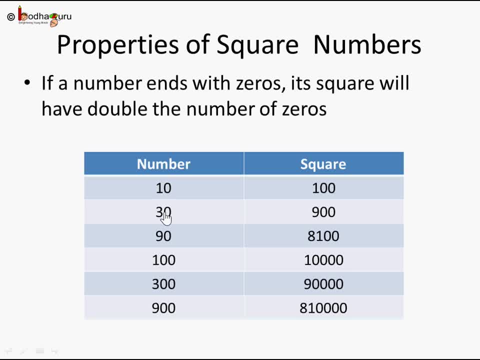 two zeros: 30, 30 square, that is 30 into 30, is 900. so here there is 1: 0 and here you see 2: 0, 90 into 90. 1, 0, here it is 80, 100, 8100 is two zeros. 900, 900 into 900 is 8 lakh. 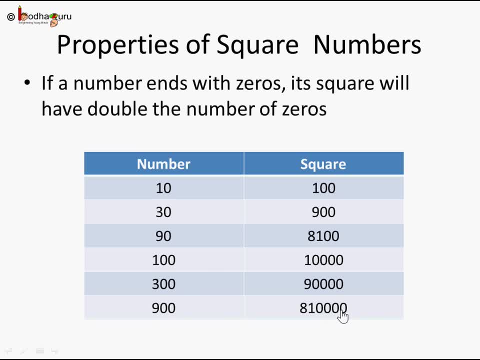 10,000. that is, here there are two zeros and here there are four zeros. so if a number has certain number of zeros- here say two zeros, or say three zeros, it's nine thousand- then it's square will have double number of zeros. so if a number has certain number of zeros- here say two- 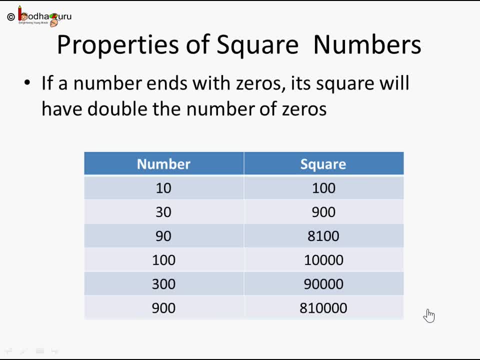 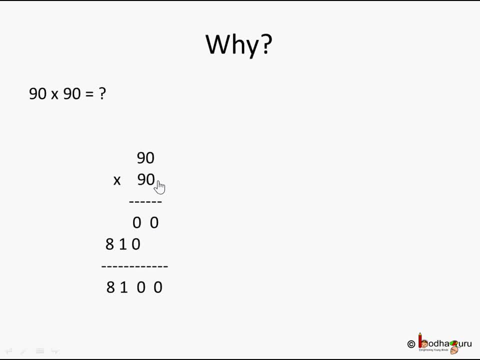 zeros, it's half zero. and if it has three zeros, then double the number of zero. so if it has three zeros here, it will become six zeros here. and why is that? same thing you do 90 into 90 in like a multiplication 0 x, anything will be 0. so 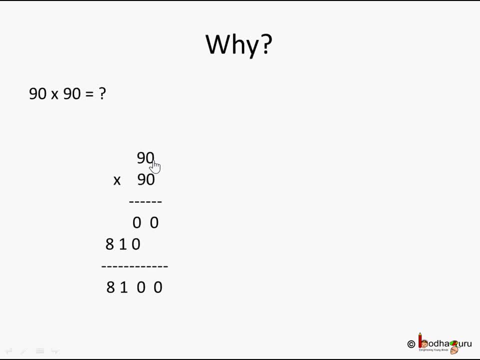 here it will be zero in the ones place. next digit also because that is 0. here, 9 into 0 is 0. so in this case, because there was one zero, one zero here, basically this will be 0 and this will be 0. you will get two zeros in the product, or it's a square. if there were 900 into 900, you will see. 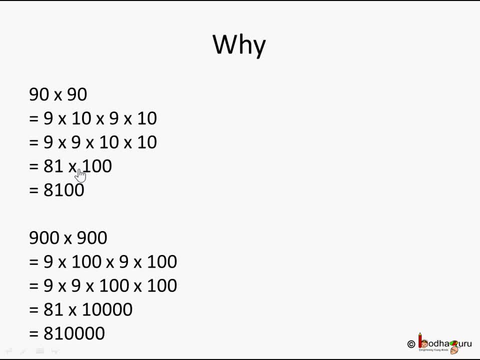 four zeros. or in other ways you can think: 90 into 90 is nothing. 90 you can represent as 9 into 10. this 90 also you can represent into 9 into 10. so it's 90 into 90, becomes 9 into 10, into 9 into 10.